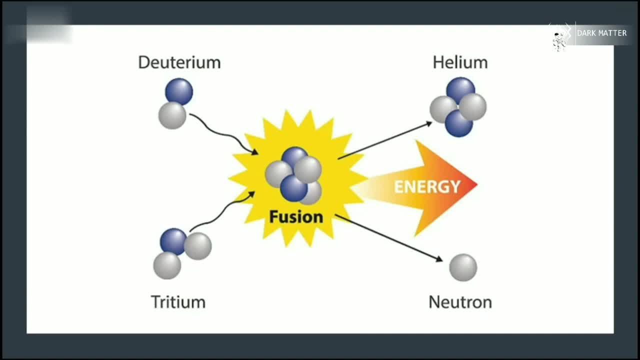 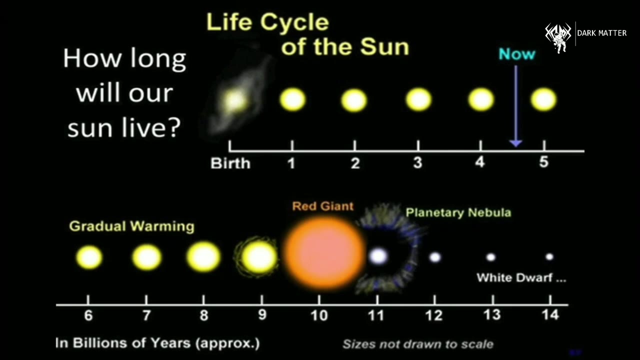 And that reaction, actually the nuclear fusion, creates a huge amount of energy, And that energy is basically the source of the energy in our sun. Now we will talk about the life cycle of the sun. So as you can see on this picture that the scales are made in a billion years. 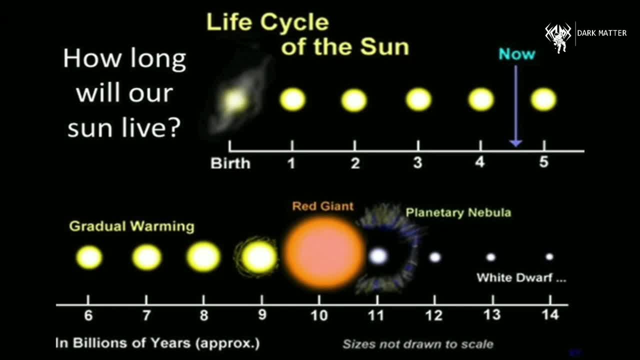 So you can see there is a now option. there is a now written between 4 and 5. So that actually suggests that the age of our sun is somewhere in between 4 and 5 billions of years, And 1 billion is equal to 100 crore. 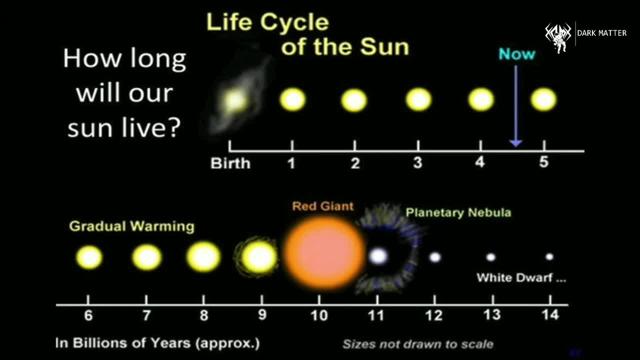 So you can actually imagine how old our sun is. And again, the total life cycle of our sun is somewhere near about 9 to 10 billions of years. So our sun will live more, few, more- 4 or 5 billion years, And after that it will become a red giant, actually it will blast and then will become a white dwarf. 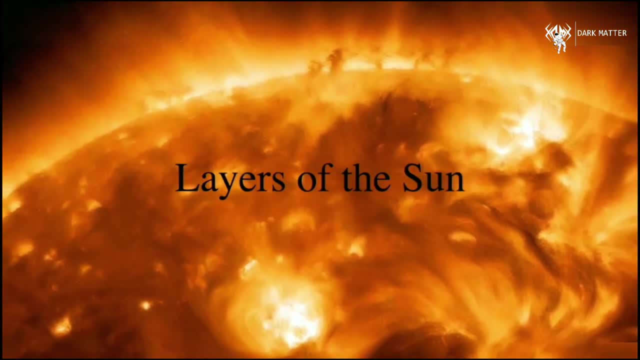 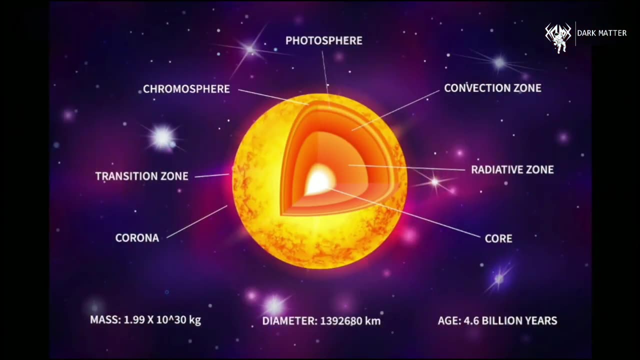 Now the layers of the sun. So inside the sun there are a few layers. Those layers are actually classified based on their temperature and some other properties as well. So the main three layers inside the sun are photosphere, chromosphere and corona. 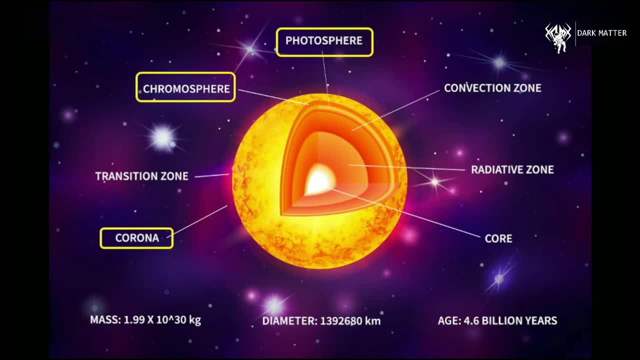 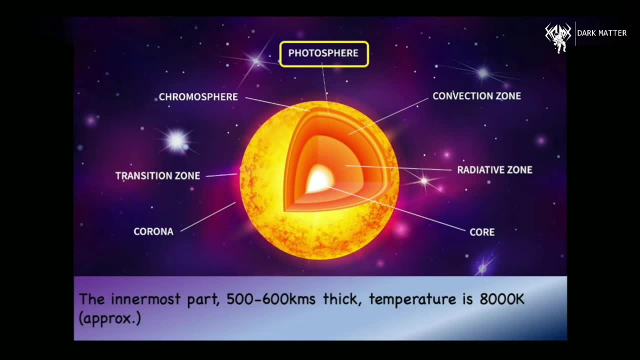 This corona is not the virus corona, by the way, Definitely that. So. photosphere: that is the innermost part of the sun, which is some 500 to 600 kilometers thick. Temperature: there is approximately 8000 kelvins. Next comes the chromosphere, which is again 500 kilometers thick. 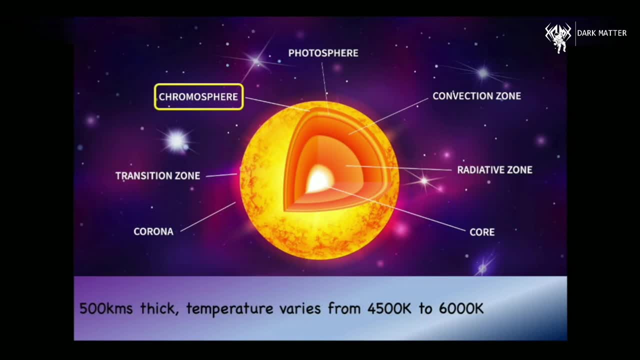 And the temperature varies from 4500 kelvins to 6000 kelvins. Now the end part, that is corona, which actually starts from the solar boundary. That is actually where the solar surface ends, From there the corona starts and it's extended by a few lakhs kilometers. 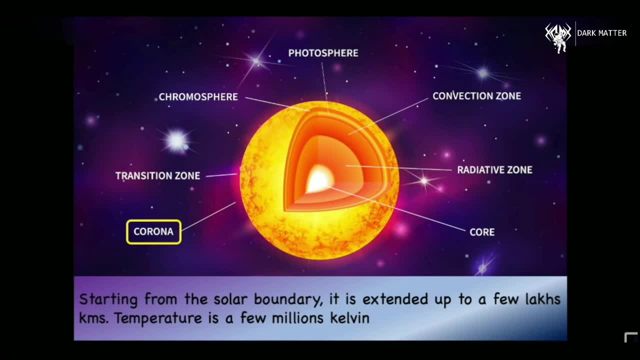 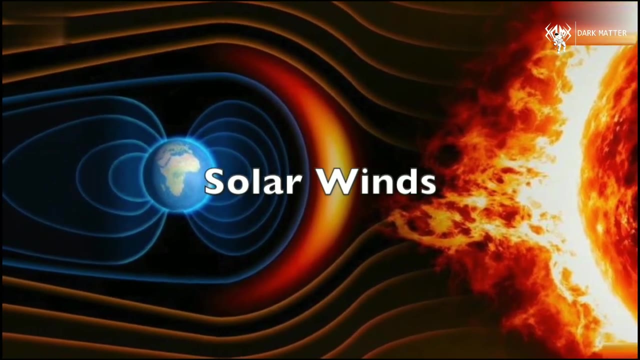 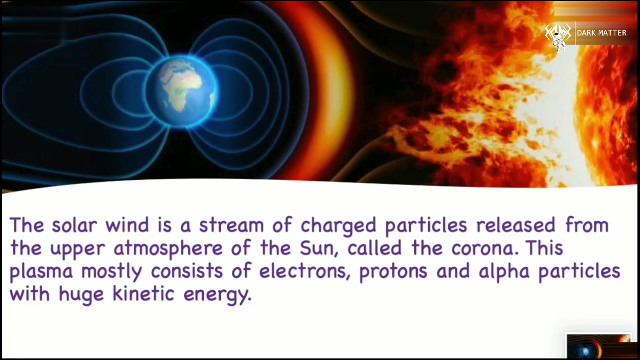 A few lakhs. The temperature there can be up to a few million kelvins. So corona is the hottest part of the sun, Solar winds. So solar wind is a stream of charged particles released from the upper atmosphere of the sun called the corona.